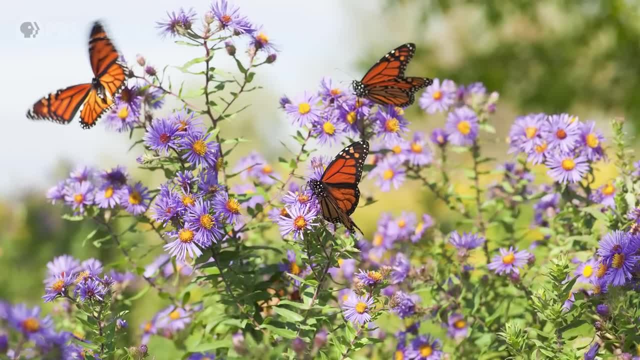 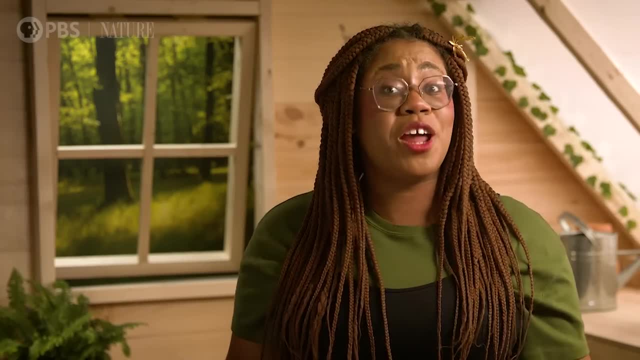 Another classic example of mutualism is between plants and pollinators like butterflies, birds and bats. They get tasty food in exchange for helping plants reproduce. And there are some lesser-known pollinator pals too. And there are some lesser-known pollinator pals too. 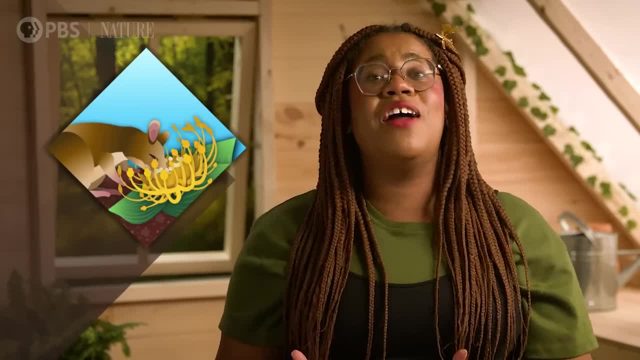 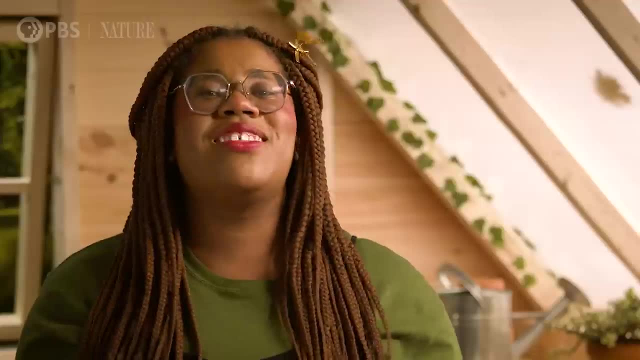 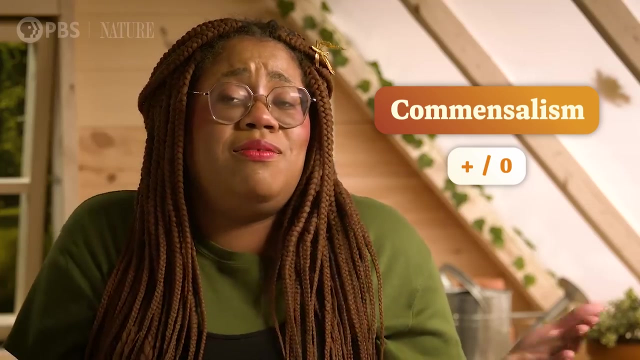 Even gerbils. In South Africa they pollinate the masonia flower by carrying pollen from plant to plant on their furry snoots. Plants can also participate in commensalism, where one species benefits and the other is just neutral. Take ferns and bromeliads, the family that includes Spanish moss and pineapple plants. 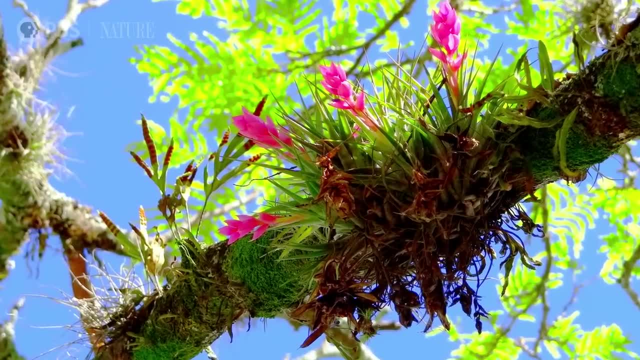 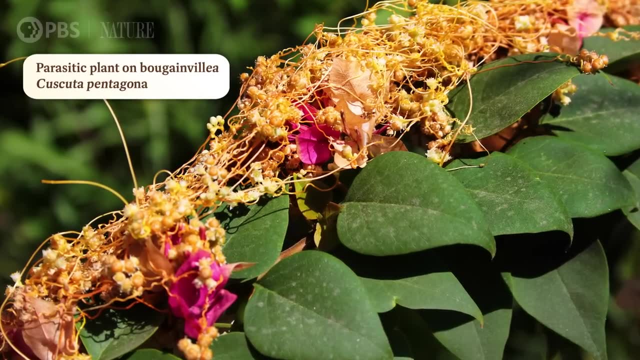 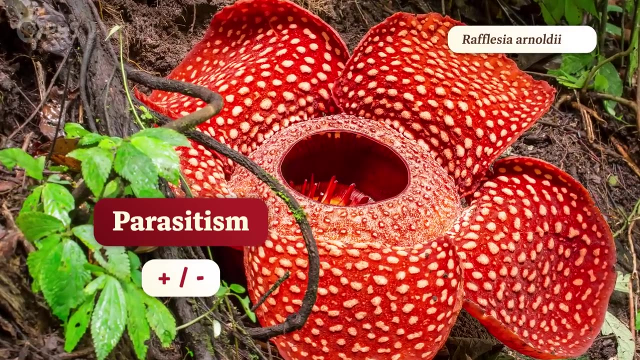 Many live on the branches of trees, and while they don't actively harm the trees, they don't do the many favors either. But not all social arrangements are good for or neutral to the plant. Many interactions are considered parasitism because the benefit to one species. comes at a cost to the other. Mistletoe, for example, is a parasite that grows high up on a tree's branches, But unlike those bromeliads and ferns which just kinda hang out on their trees, mistletoe sucks water and nutrients from its tree, which can stunt its growth. 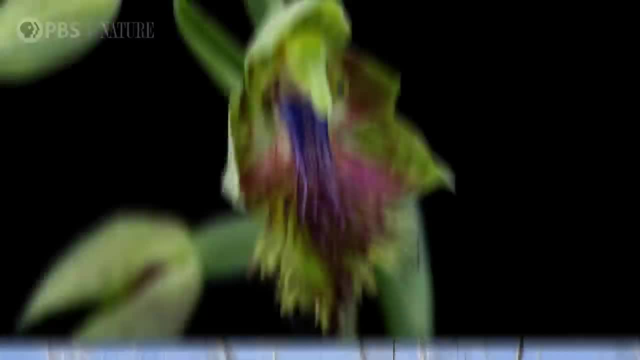 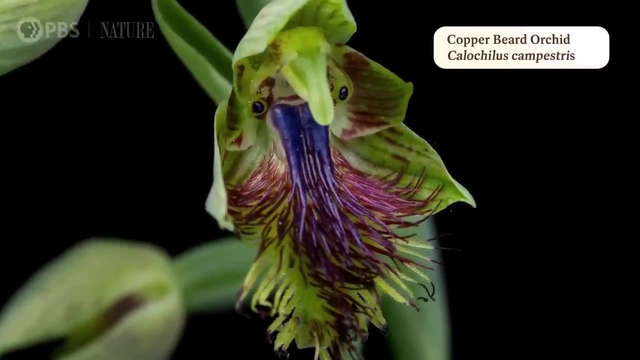 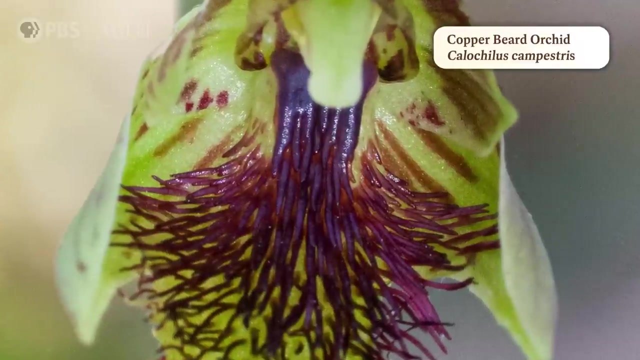 Not exactly a Hallmark movie moment. Even those plant-pollinator interactions can sometimes head into parasitic territory. There's an orchid that mimics the shape and scent of female wasps, so male wasps waste valuable energy and sperm trying to mate with it. 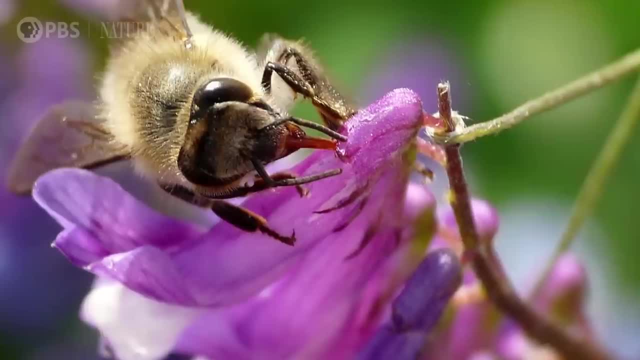 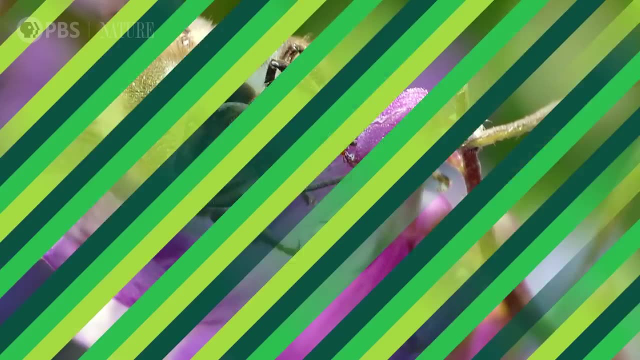 while the plant reaps the benefits of pollination, And there are insects that rob nectar from flowers without transferring any pollen at all. Think of how cherries end up burning their leaves. Talk about some toxic friendships. And so you can always keep some pollinators out and you have the opportunity to see them get. to the root of the plant details. Ramble, ramble, ramble, ramble, Murmiding as they walk around a branch of a tree. Sit and look around for its yet unfinished branch, Tempting the big-اصle. and the ants droop their hatches. Don't forget that money will notvet. a fresh bunch of wasps are a good thing. 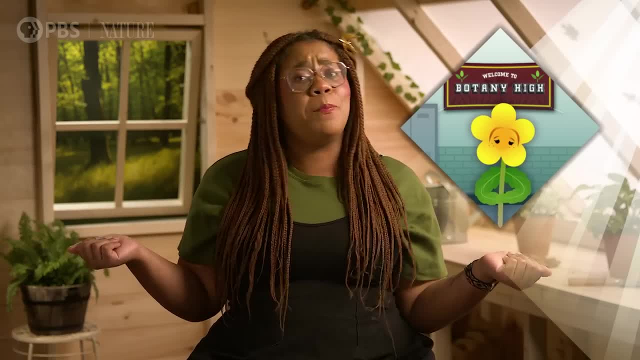 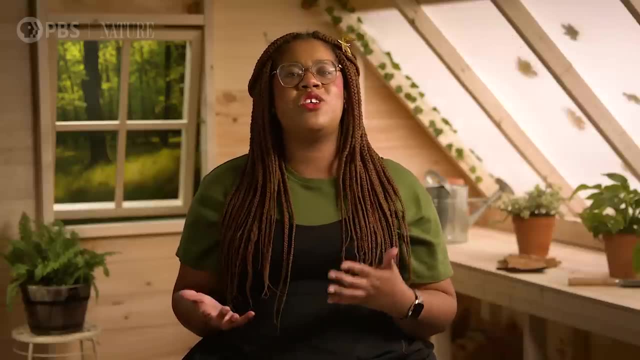 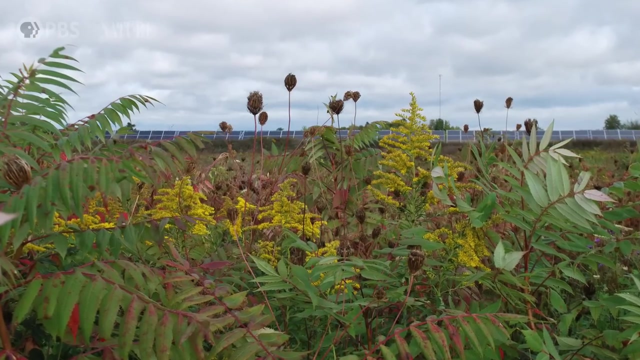 Understanding all of these different interactions isn't just useful for a plant teenager trying to survive botany high. it's also crucial to conservation or the protection of species diversity from threats like climate change and habitat destruction. After all, we can't restore wildflower meadows without their pollinators and saving rare 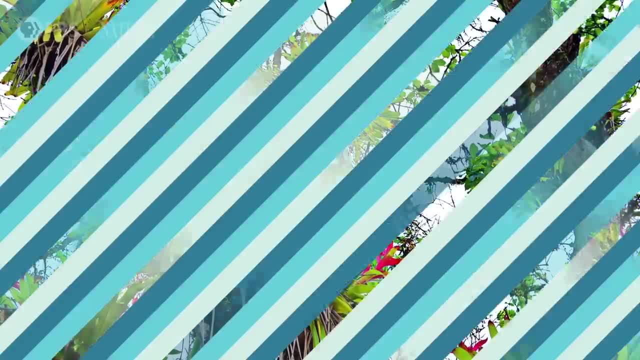 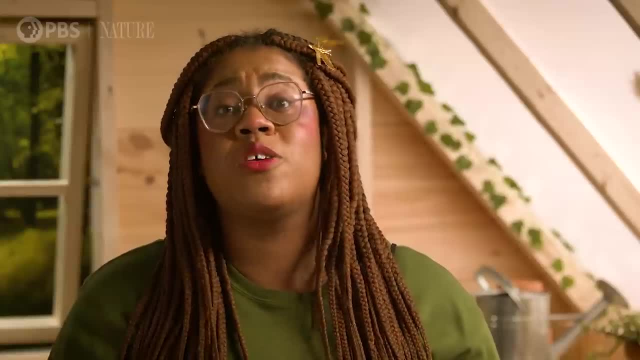 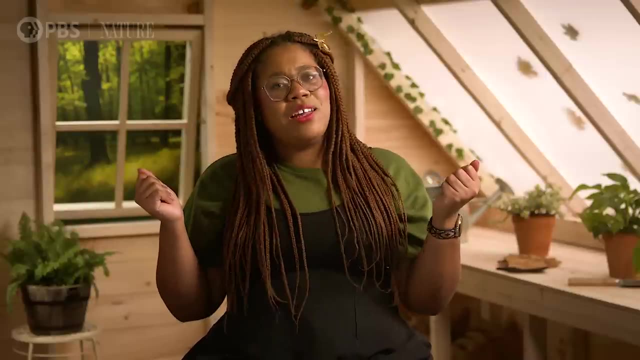 bromeliads can't happen if there are no trees for them to grow on. In other words, all plants are connected to other organisms, so conservation has to consider those networks of relationships. Anyway, now that we've covered the scale of one-on-one interactions, let's zoom out. 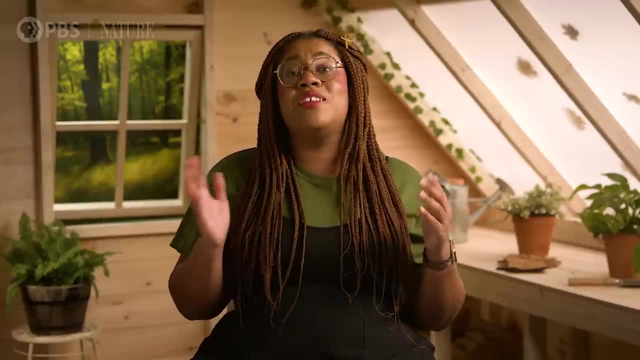 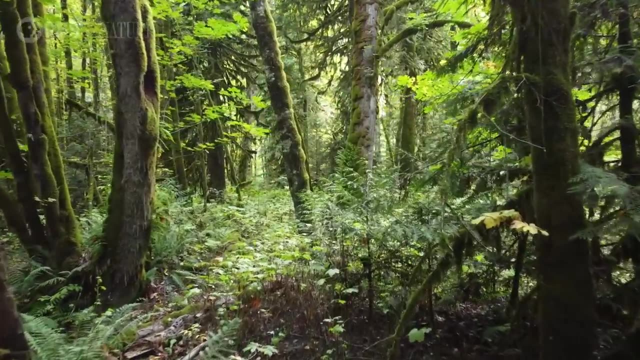 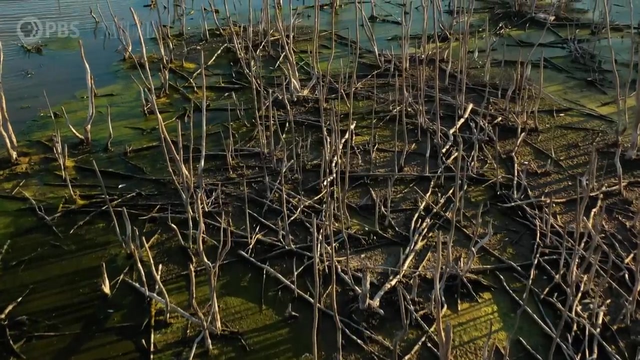 a level to look at groups of the same species living in the same place, In other words, populations. Populations change over time. they grow or shrink, they rearrange themselves into different patterns or distributions, and often these changes are influenced by environmental factors. 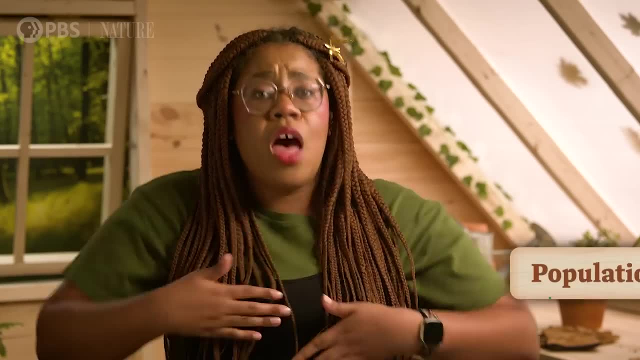 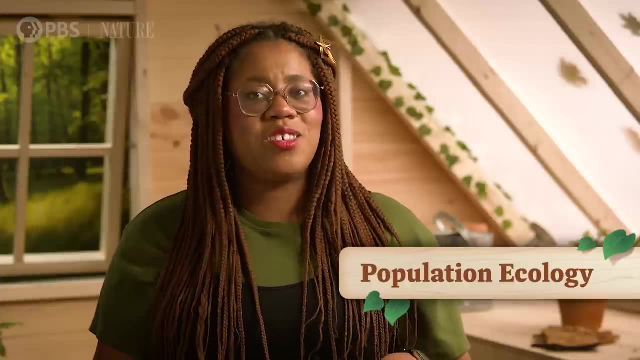 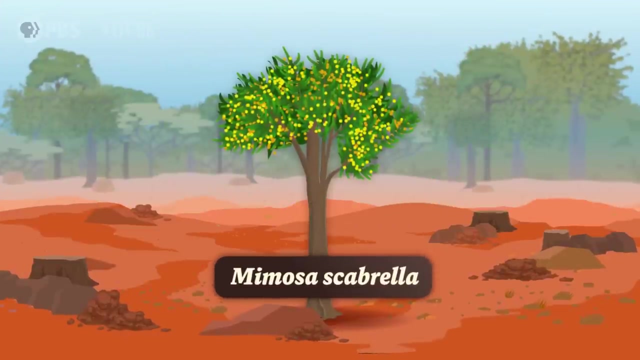 These shifts and the forces that trigger them change over time, And by studying these types of population changes, population ecologists can learn things that go beyond a single species. Take Mimosa scabrella, a species in the pea family that's native to Brazil. 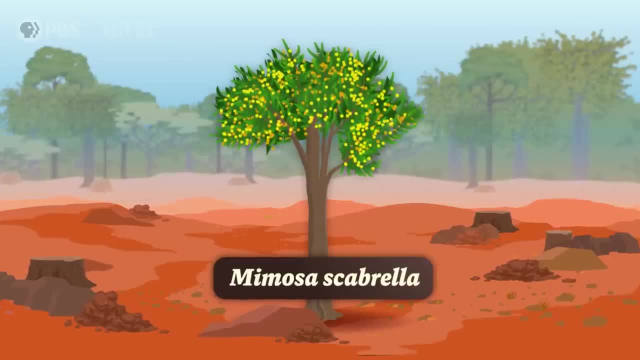 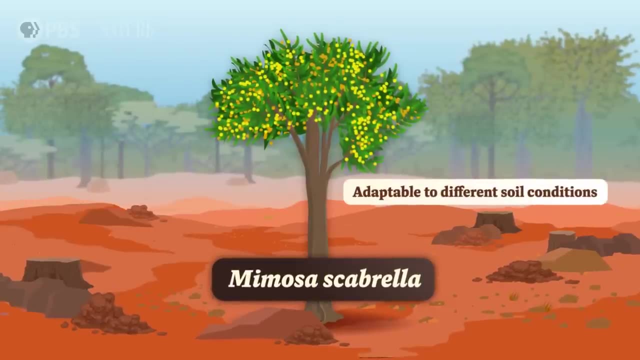 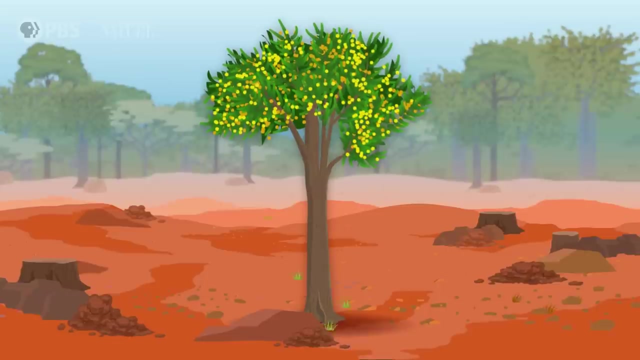 It tends to be one of the first species to regrow in areas that have been disturbed by harmful human activity. That's because the tree is super adaptable to different soil conditions, even though it has been depleted by things like mining, And as it begins to regrow, the plant makes the area more hospitable for other species. 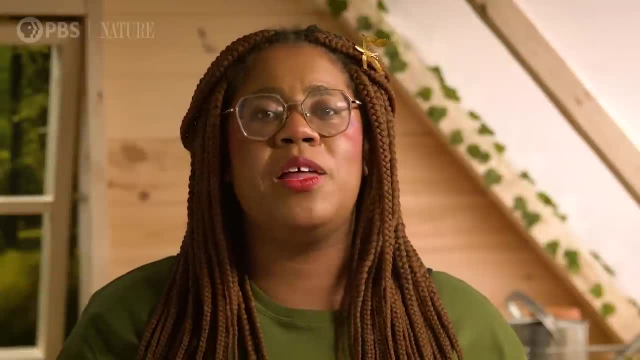 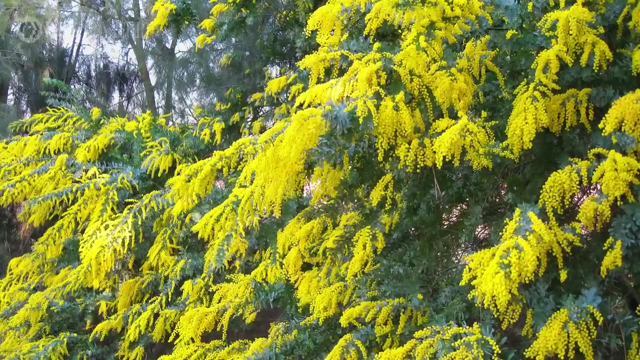 to do the same. So the distribution and abundance of this population in a damaged area is a good indicator of how well the area is recovering overall. But while Mimosa scabrella is a conservation hero on one hand, it presents conservation challenges on the other. 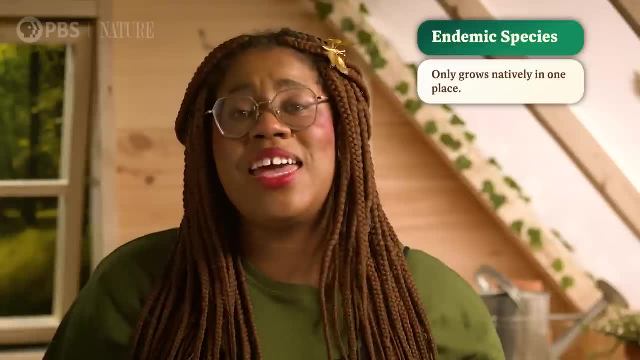 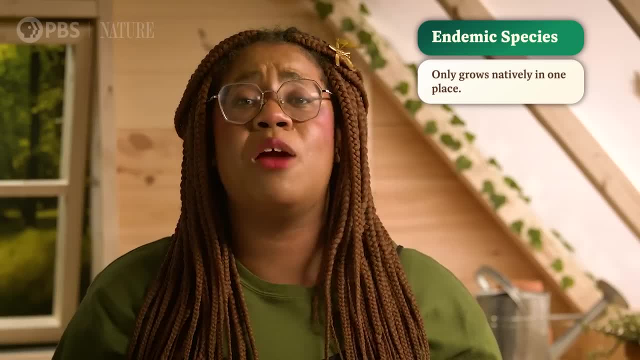 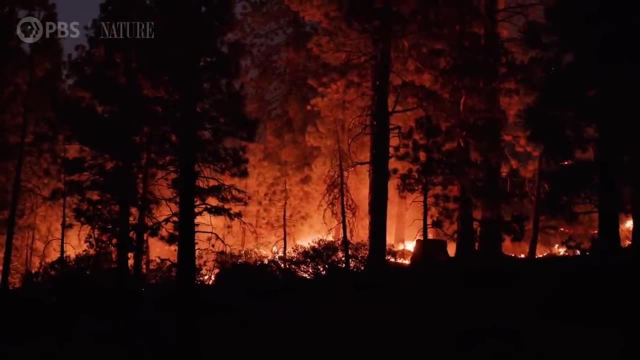 It only grows natively in one place, making it an endemic species. It only grows natively in one place, making it an endemic species. An endemic species are particularly vulnerable to environmental changes or events. Think about it: For widespread species, a forest fire might wipe out a local population. 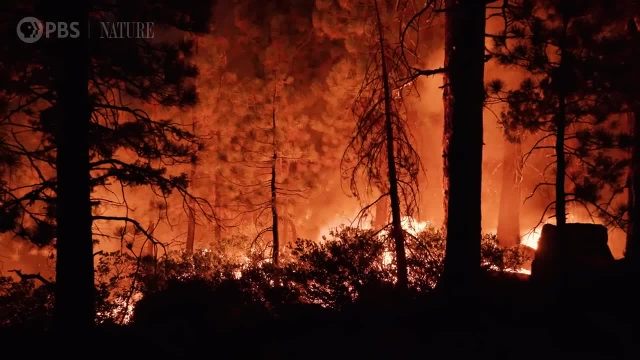 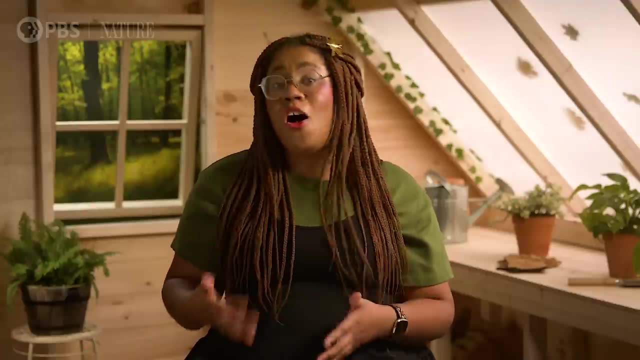 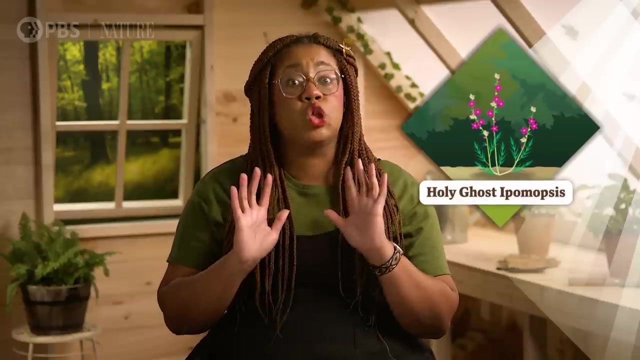 But for an endemic species that wiped out population might be the entirety of the species. So population ecologists monitor and sometimes alter populations for conservation purposes. Like the Holy Ghost, Ipomopsis is a particularly vulnerable species. Like the Holy Ghost, Ipomopsis is a particularly vulnerable species. 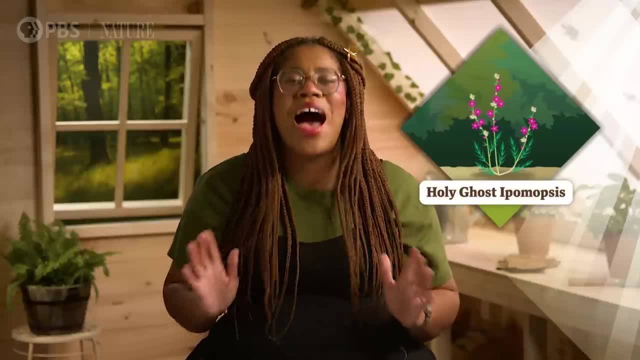 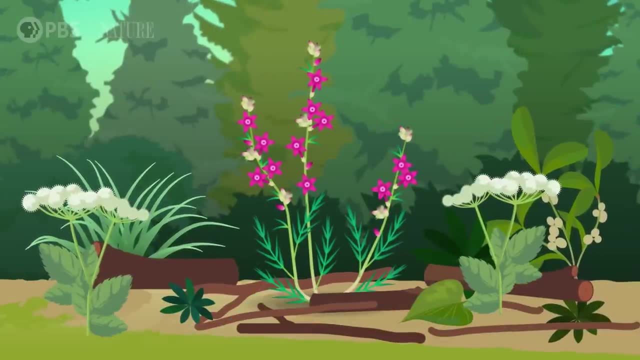 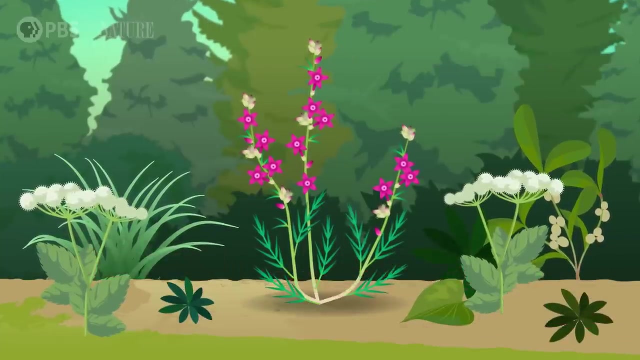 This homebody is endemic to only a two-mile stretch of a canyon in New Mexico, And ecologists are using two strategies to conserve it. One is in situ conservation, which takes place in the plant's native habitat and involves clearing debris that could fuel forest fires and trimming back other plants that are encroaching. 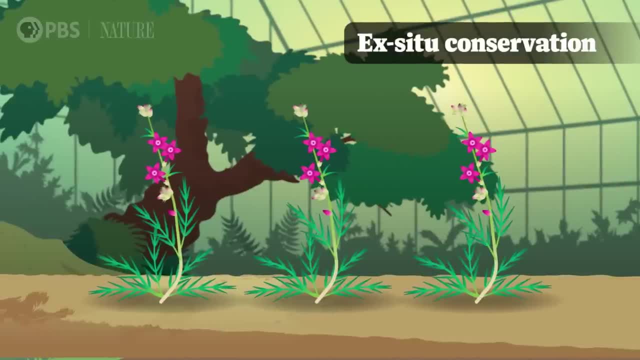 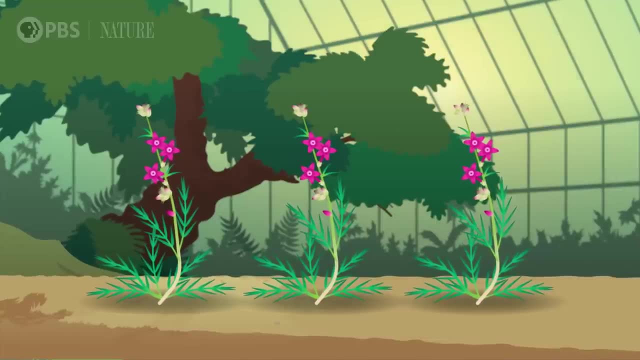 on the Ipomopsis territory, The other is ex situ conservation. The other is ex situ conservation, The other is ex situ conservation, Where new populations are started outside the species' natural habitat. Botanists are growing lots of Ipomopsis in botanical gardens, so the species won't be 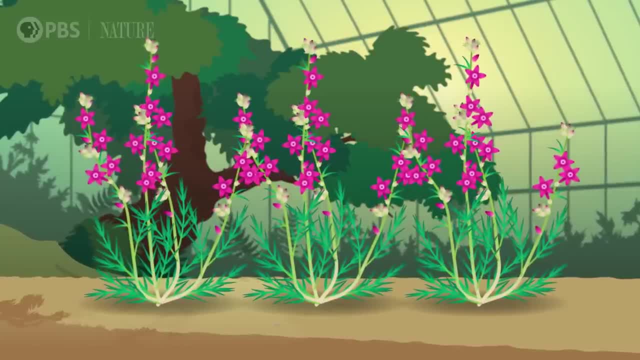 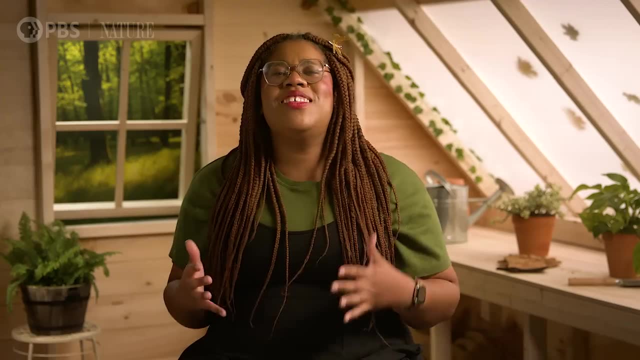 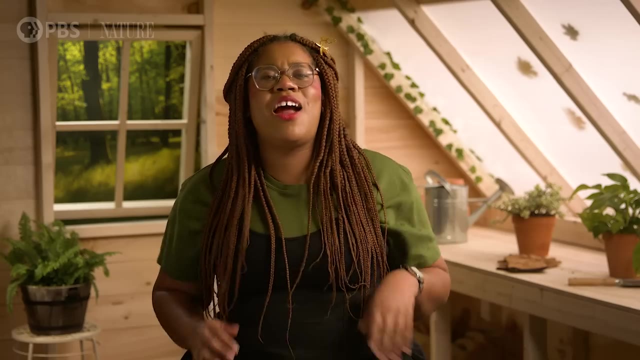 lost to a disaster. And once the plants grow strong, the ecologists reintroduce some of them back to their native habitat in an effort to expand the population. So we can study individual species through population ecology, But we can also zoom out one step further to consider how groups of different species 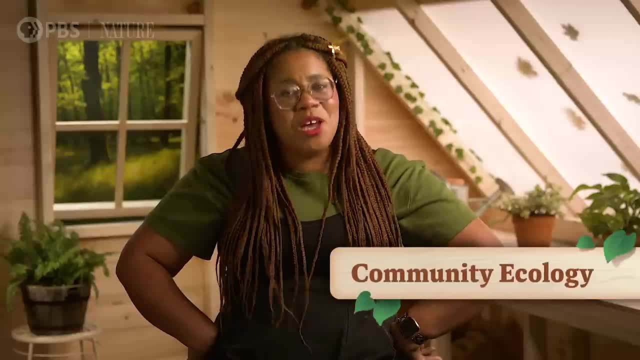 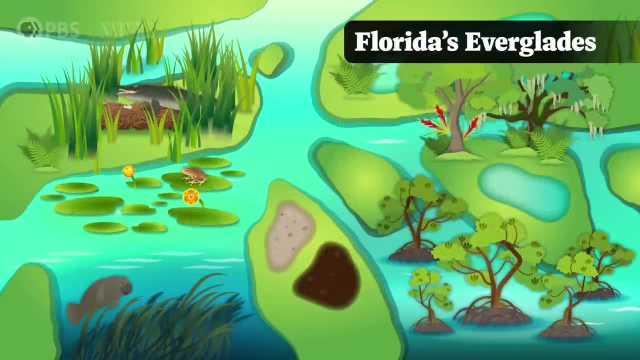 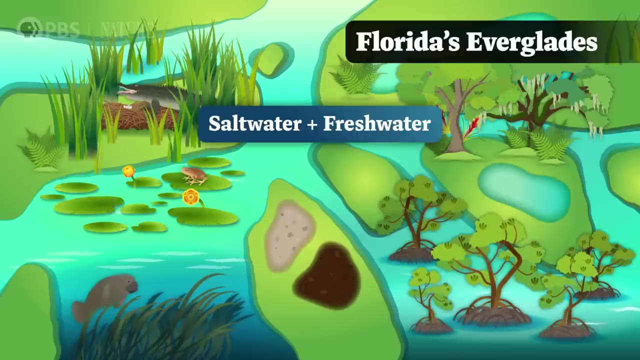 interact in a shared space. This is the focus of community ecology. To witness community ecology in action, let's head to the Thought Bubble. Welcome to Florida's Everglades, one of the world's largest wetlands. Its combination of salt and freshwater, varied soil types and subtropical climate has led 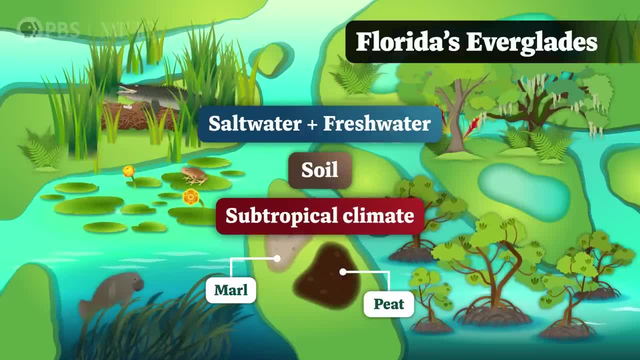 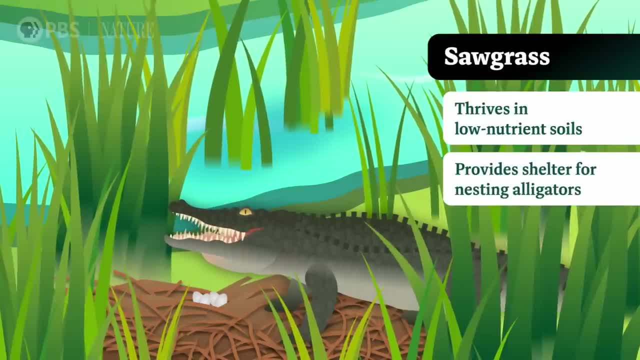 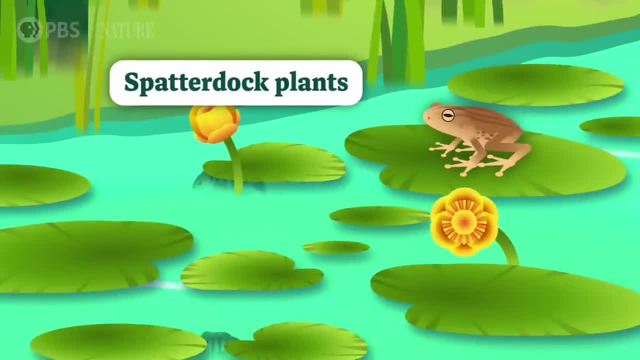 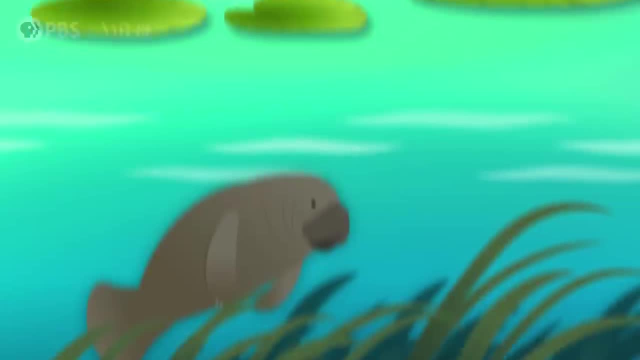 It's a great place to be. I respect you from a distance. large lizards. Then there are ooh Spattered dock plants which provide cover for frogs and fish and whose seeds are eaten by ducks. Yum, Underwater manatees feed on seagrasses. 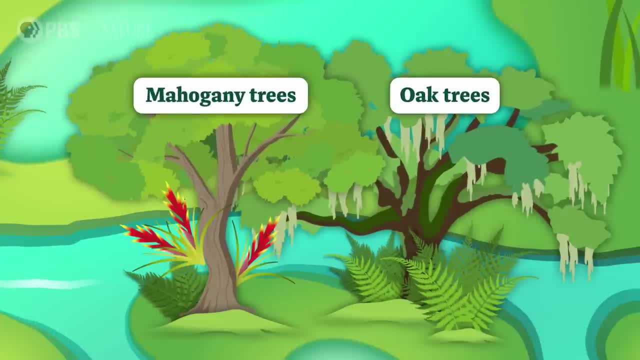 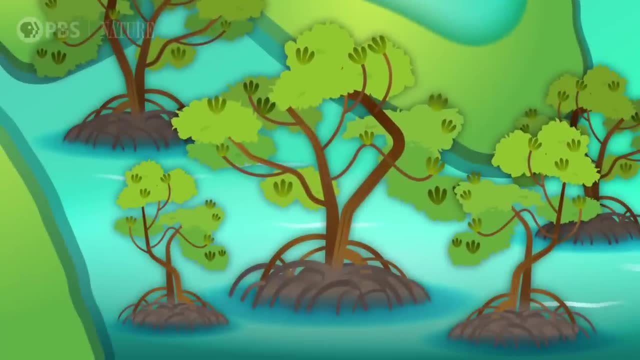 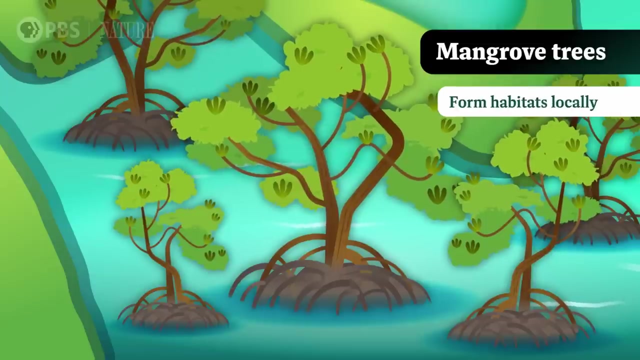 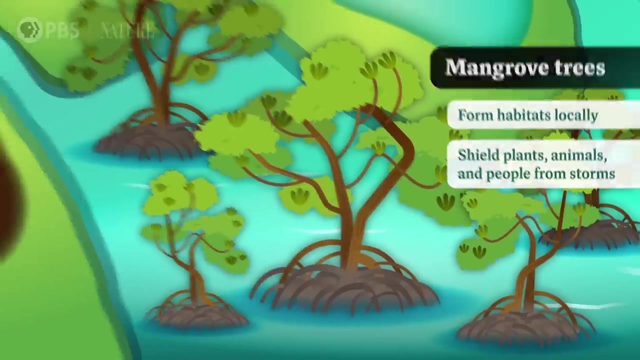 And on land. mahogany and oak trees provide a habitat for other plants to grow, like bromeliads and ferns. On top of that, the Everglades are home to the largest mangrove tree population in the Western Hemisphere, which not only form habitats locally, but also help shield those inland plants, animals and people from storms. 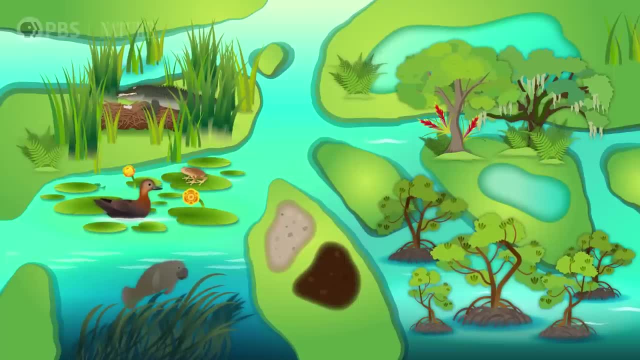 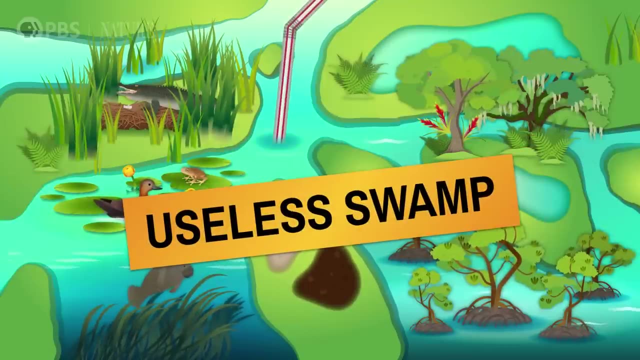 But in the early 1900s nobody really knew about this complex community. Most Floridians thought that area was a useless swamp and developers started to drain it so they could build on the land. Enter the journalist and activist Marjorie Stoneman Douglas. 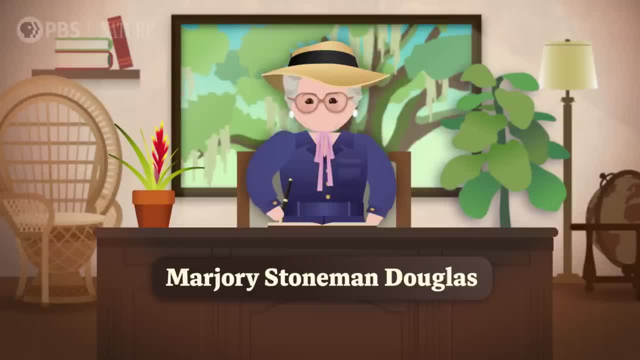 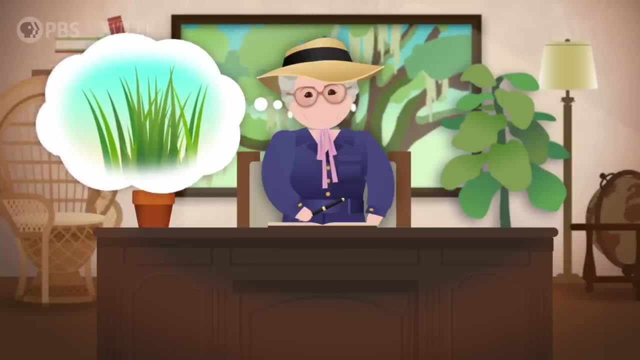 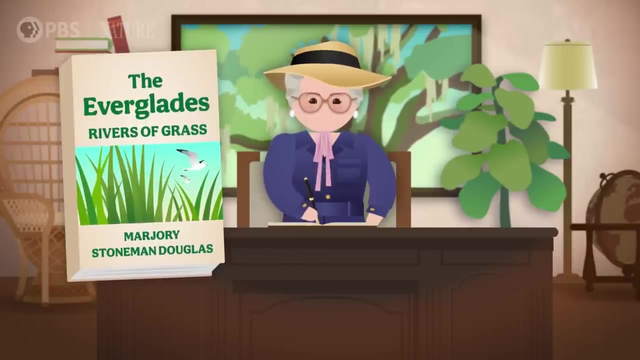 In her later years, Douglas was determined to save the Everglades. She wrote articles and published a book that was kind of a love letter to the swaying sawgrass we saw before. Her writing made a huge impact on public opinion and Floridians began to recognize the value of this ecological community. 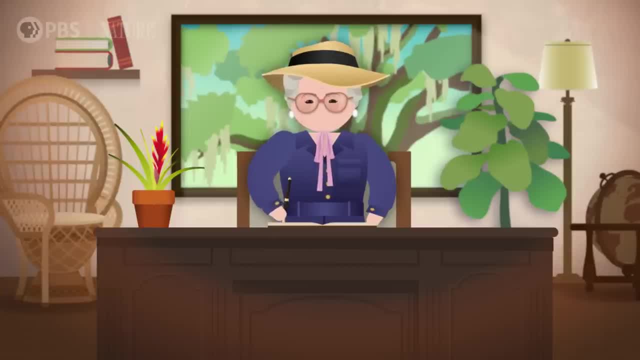 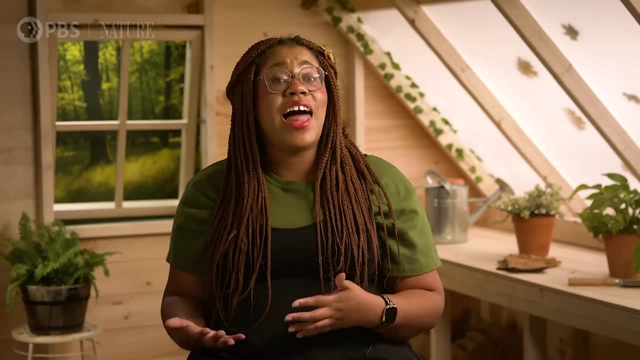 And in 1947, the Everglades National Park opened, which formally protected it, And in 1947, the Everglades National Park opened, which formally protected it. Thanks, Thought Bubble. So plants live their lives in the larger context of communities and they can play huge roles in shaping their environments. 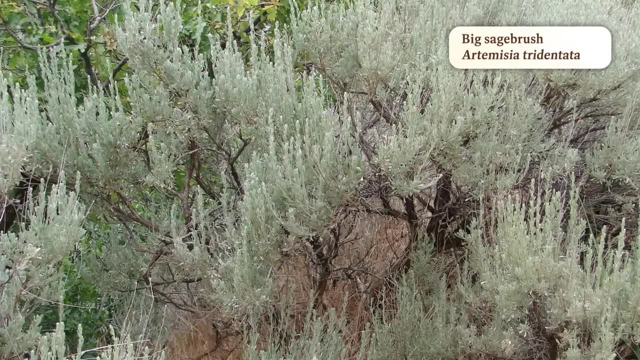 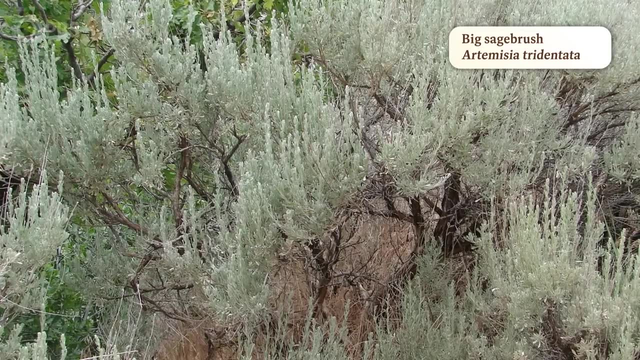 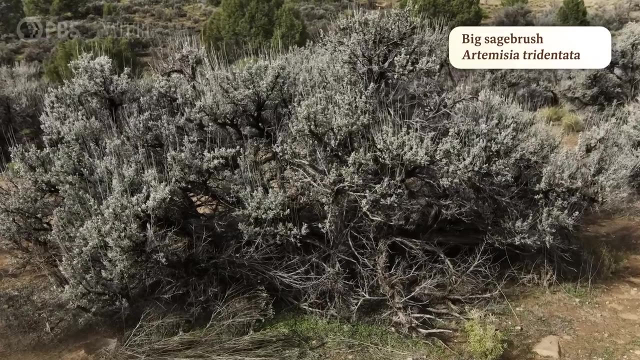 Like one plant species might help others grow more by making the environment less harsh. Community ecologists call this dynamic facilitation, and the big sagebrush plant is a pro at it. In North America's deserts, water is pretty scarce, which is a challenge for plants. with shallow roots. But when big sagebrush sends its super deep roots far into the soil to search for water, it brings that water up to the shallow-rooted plants as well. On the more dramatic side of things, plants also engage in competition. 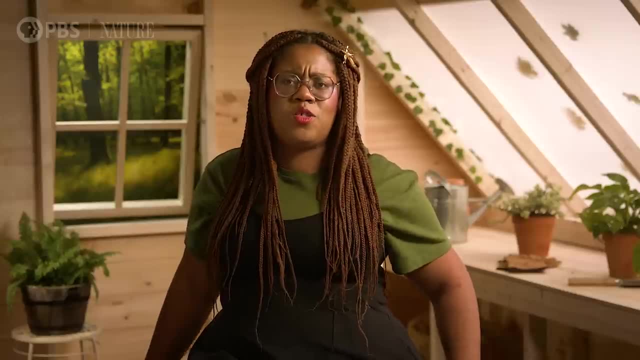 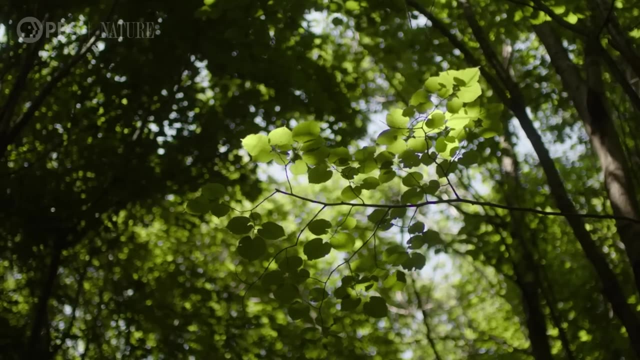 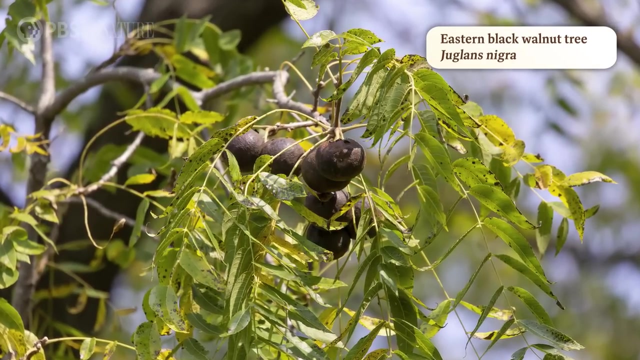 where they make the environment more difficult for other species to survive. Most plants compete with each other for light and nutrients. A little healthy competition isn't so bad. But some plants secrete chemicals from their roots into the soil to prevent other species from sprouting nearby. 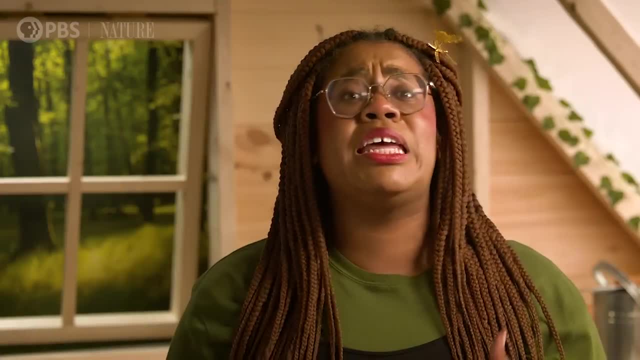 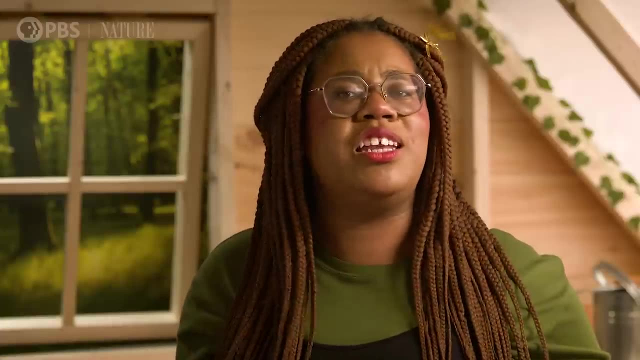 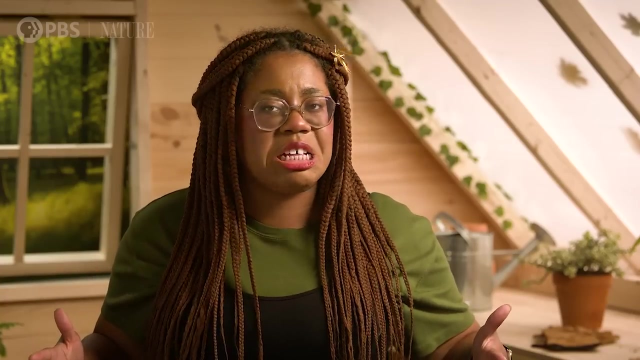 And that is a little more cutthroat And competition can get really out of hand when invasive species or species from another area come onto the scene and totally disrupt ecological communities. For example, a major invader in the western US is cheatgrass. It was introduced to the region accidentally in the 1800s. It's likely because its seeds got mixed in with other agricultural products. Now, you see, the problem is it grows back after the winter thaw earlier than the native species do, so it sucks up the water supply first. 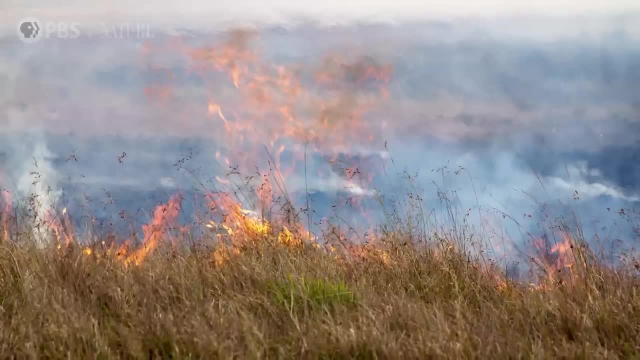 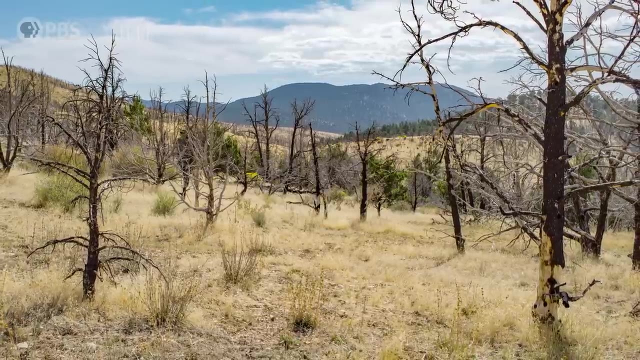 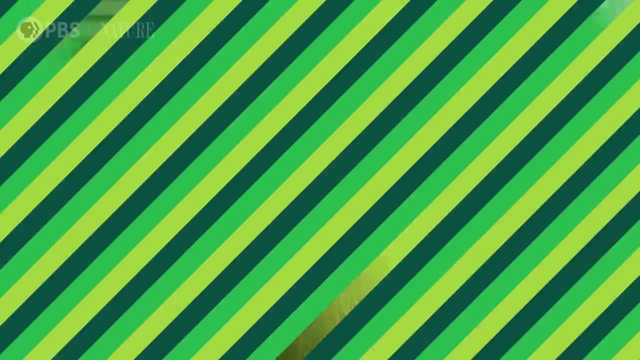 Those meanies. It also produces a lot of plant material that can become fodder for fires, And it can re-sprout super fast even after a fire rolls through, So it quickly dominates the habitat and pushes out native species. This has huge effects on the ecological community. 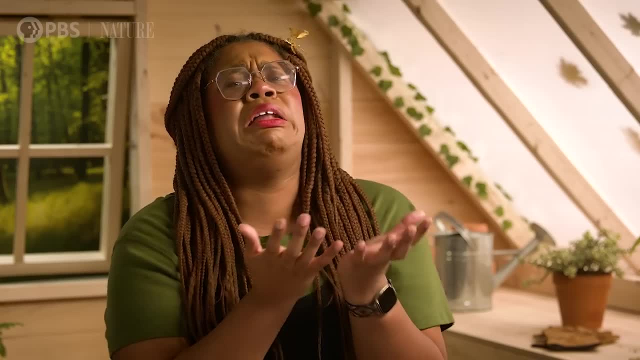 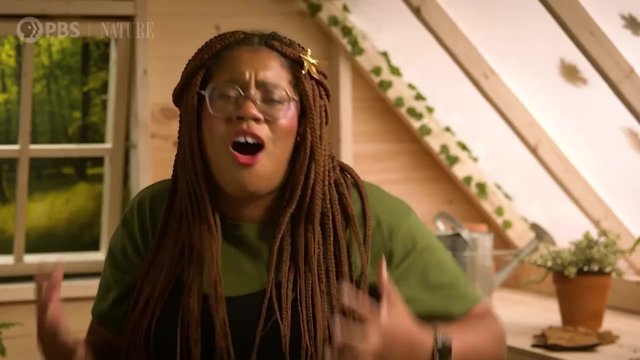 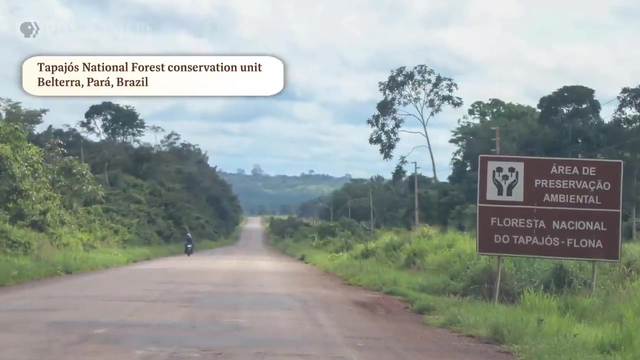 Delicate relationships are disturbed, soil is degraded and essential nutrients are intercepted. This all makes it harder to restore the area after it's been disrupted. The good news is there are many conservation efforts happening worldwide to protect plant communities from threats like habitat loss and the effects of climate change. And at the local level there's a lot of work to be done. Your country's Forest Service likely provides resources on how you can reduce harm from invasive species in your own community. This might involve things like removing contaminated soil Or even digging up the plants themselves.